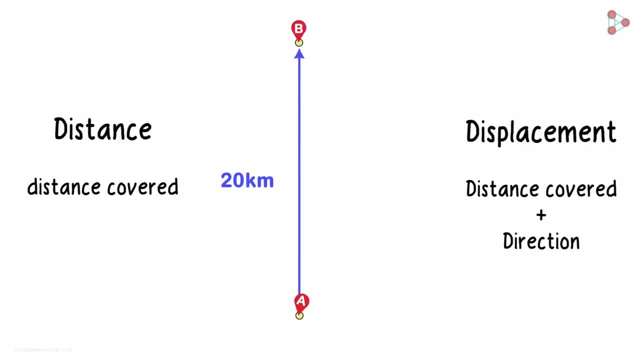 Say, the distance between towns A and B is 20 kilometers. So if we take a 50 kilometer route from point A to B like this, then the distance covered is 50 kilometers and the displacement is 20 kilometers north of point A. 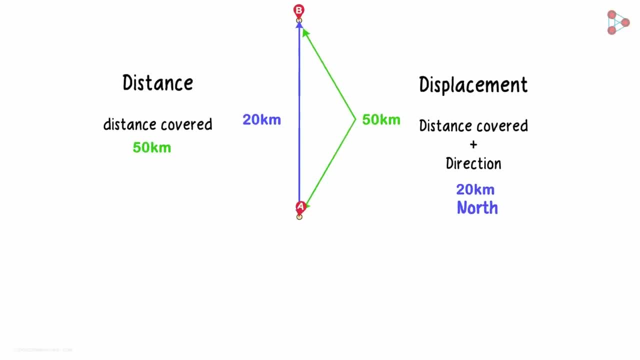 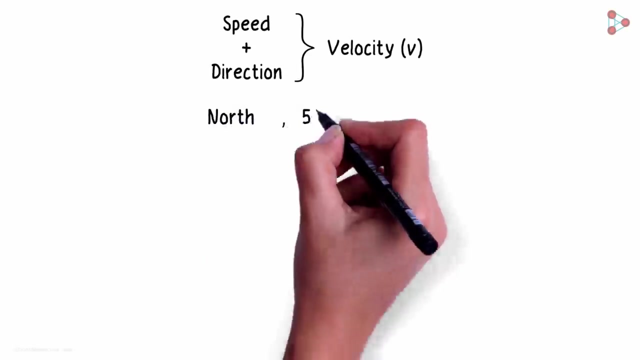 So speed does not tell us the direction. Is there anything that tells us the speed along with direction? Yes, it's velocity, which can be written as lowercase v. Let's see how it differs from speed. What if I tell you that I travelled north at a speed of 50 meters per second for one minute? 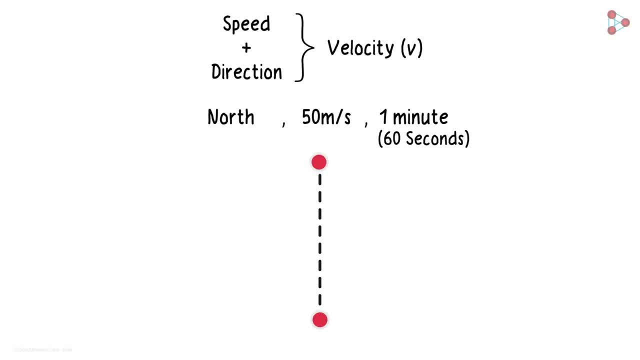 Would you be able to tell me where I landed up? Yes, you would know. I have covered a total distance of 3000 meters and landed up at this point. Velocity is speed with direction of motion. As such, velocity is direction aware. 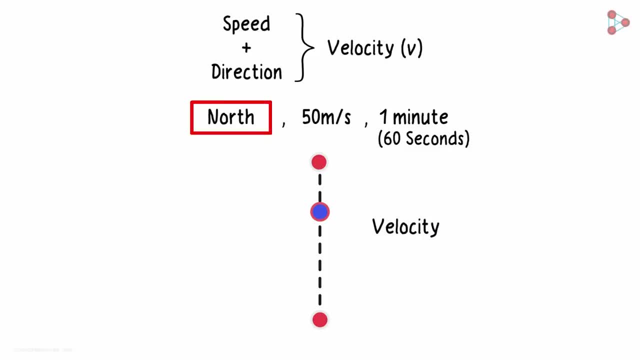 So when you mention velocity you must keep track of direction. Something like the car moved south at 55 miles per hour. If you do not mention the direction and just say the car moved at 55 miles per hour, you are not stating the velocity anymore. 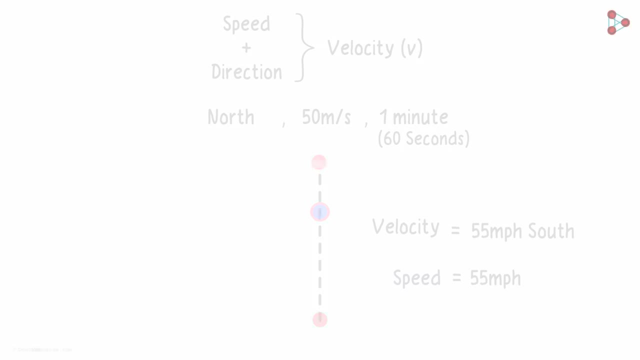 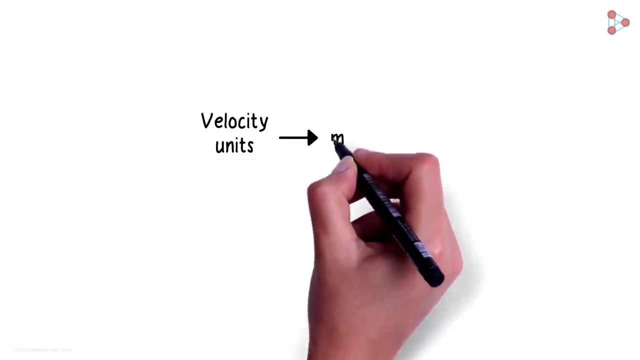 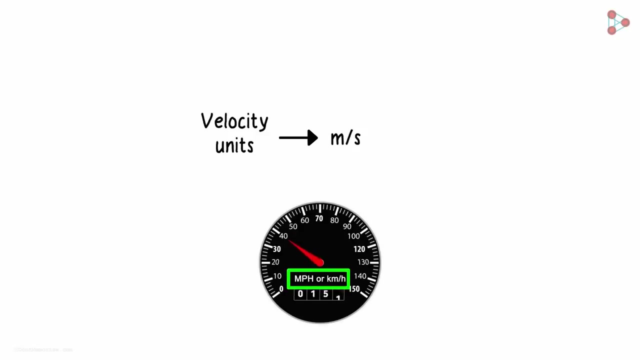 What you are stating is the speed. What do you think is the unit of measurement for velocity? The unit of measurement for velocity, just like speed, is meters per second. Now you might ask: why meters per second? The car's V-drive indicates speed in miles per hour or kilometers per hour. 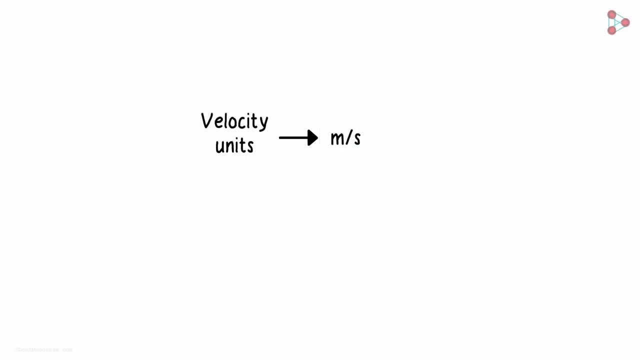 So why is the unit for velocity meters per second? The established SI unit of measurement for velocity is meters per second, And SI stands for International System of Units. This helps everyone in the world adhere to velocity. This is one common style of measurement. 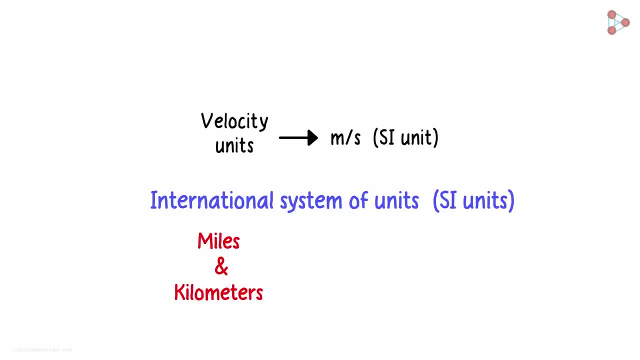 Imagine the confusion created with different measures like miles and kilometers, gallons and liters, US gallons and imperial gallons, etc. Incidentally, speed and velocity are both measured in meters per second, But do you remember which one is a scalar quantity and which one is a vector quantity? 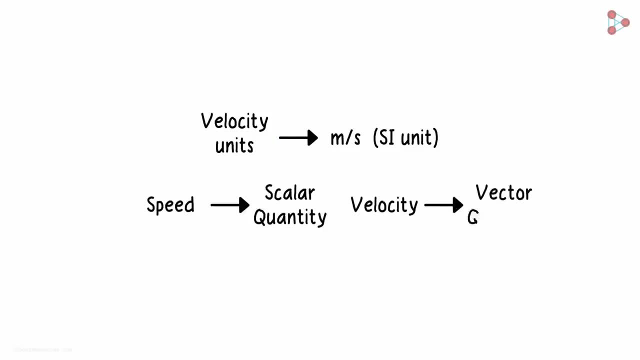 Yes, speed is a scalar quantity and the velocity is a vector quantity, as the direction is also specified. Now let me ask you an interesting question: What is average velocity? To make it a bit easier for you, let's look at the example we looked at in our first video on motion. 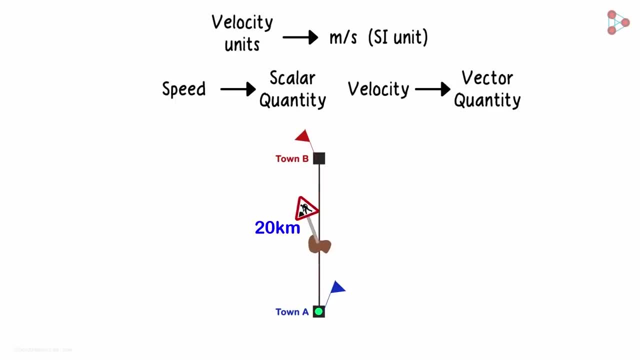 You have to travel 20 kilometers up north, But because of the road works, you took an alternative path which totaled 50 kilometers and you took 2 hours to reach the destination. This was your path of travel. Let's make two columns here. 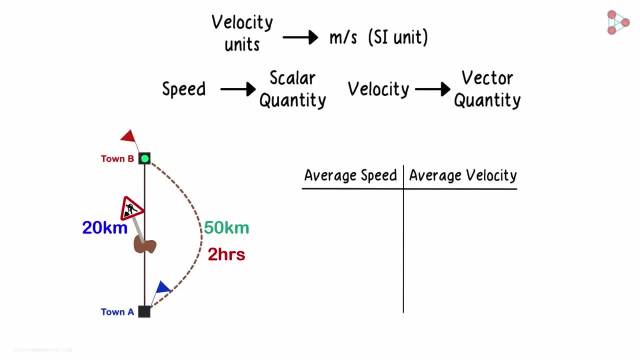 One for average speed and another for average velocity. Do you remember how we calculated average speed? Yes, it is the total distance covered over the total time taken. So 50 over 2 will give us 25 kilometers per hour as the average speed. 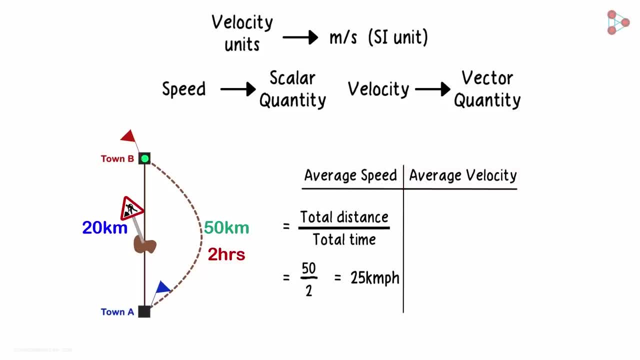 Now, what will be the average velocity here? The average velocity depends only on the start and end points, regardless of path taken. Do you remember we had learned about displacement? So the average velocity equals displacement over time. What is the displacement here? It's 20 kilometers up north. 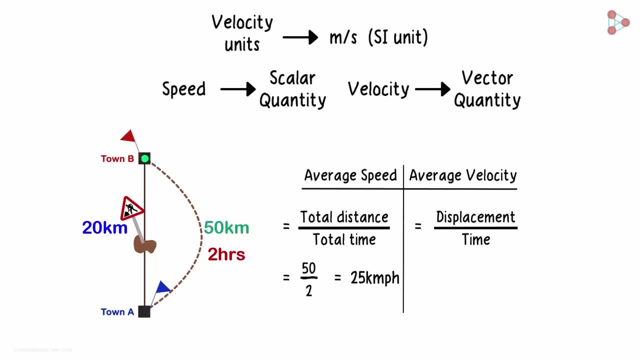 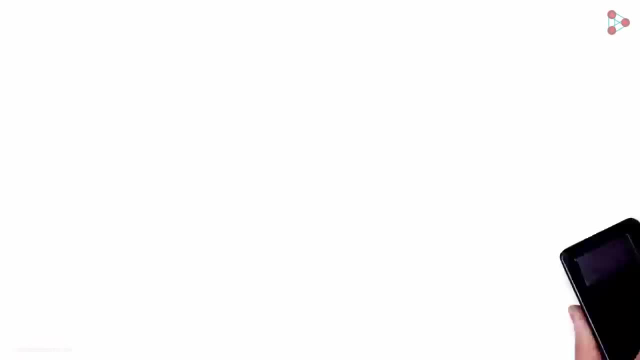 Distance with direction. So the average velocity will equal 20 kilometers over 2 hours, which will equal 10 kilometers per hour. That's the concept of average velocity. So if you think you've really understood this concept, here's a question for you. 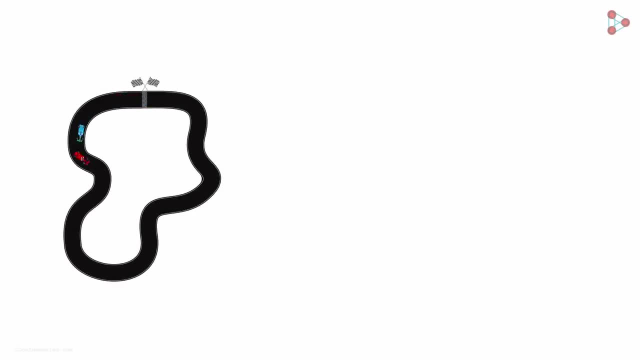 You are a Formula 1 race car driver. You had a great race and finished the 300 kilometers race in 1 hour and 40 minutes at number 1 position. What was your average velocity? Ok, if you didn't get it, let me give you a hint. 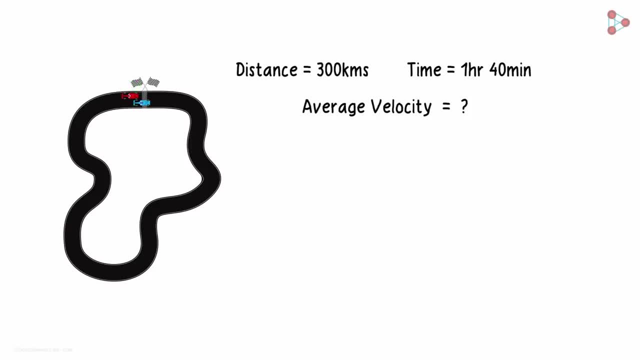 This was your start point and finish line as well. They were both the same. You went around the track several times, only to eventually finish at the same point where you started. So tell me now what was your average velocity? First, can you tell me what your displacement is? 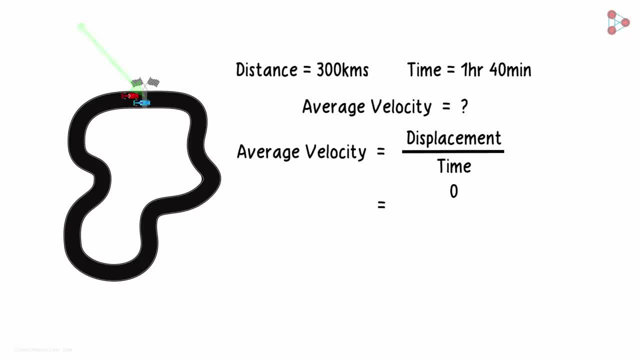 You started and finished at the same point, So your displacement is 0.. 0 divided by the time taken, which is 1 hour 40 minutes, equals 0.. That puts your average velocity for the race today at 0 meters per second.